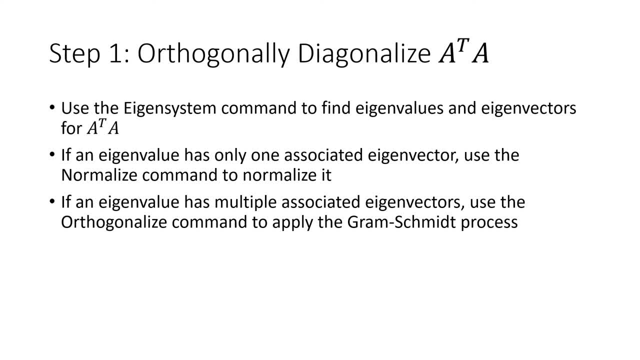 diagonalizable. That means that it's diagonalizable and we can find a full basis of eigenvectors for our full space Rn. that consists entirely of eigenvectors that are orthogonal to each other and are all also unit vectors, A so-called orthonormal. 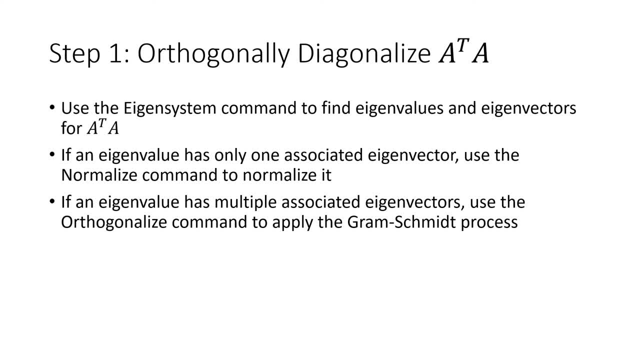 basis for Rn. So the way that we're going to do that is by using the eigensystem command. That's going to give us a list of eigenvalues and eigenvectors associated with those eigenvalues. But those eigenvectors that we get will not necessarily be unit vectors and they won't. 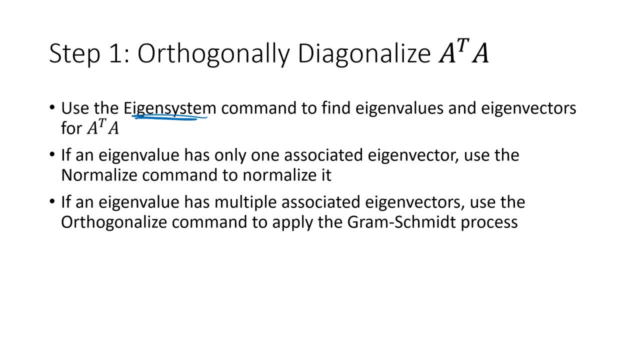 necessarily be orthogonal to each other. So the way that we're going to fix those eigenvectors is either by normalizing them. So normalize: just takes a vector and either shrinks it down or expands it out to be a unit vector. That's what we're going to do if we only have 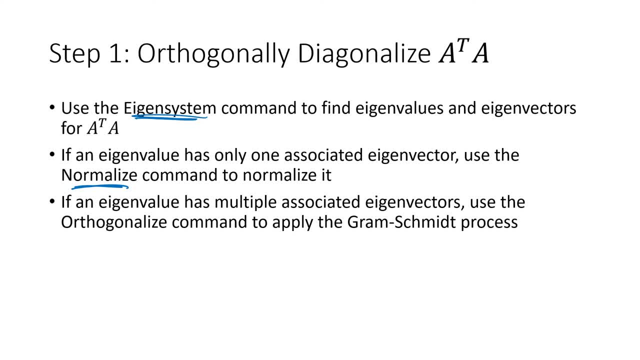 one eigenvector associated with a given eigenvalue. But if we have multiple eigenvectors associated with a given eigenvalue, we need to not only make them be unit vectors, but we need to make them be orthogonal to each other, And so for that, we're going to use the orthogonalize command, which does the 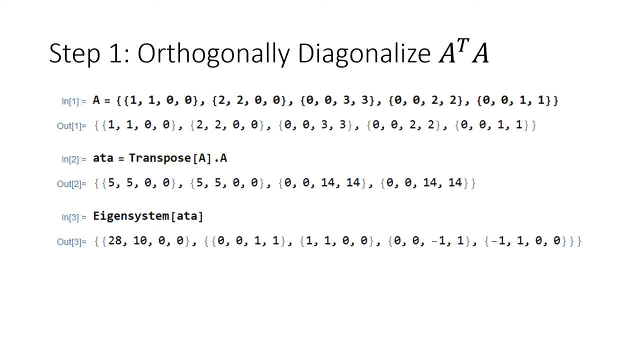 Gram-Schmidt process to make those vectors be orthogonal. So here's what this is going to look like for our matrix A. So the first thing that I'm doing here is just typing in the matrix A. The next thing I'm doing is defining the matrix A transpose. 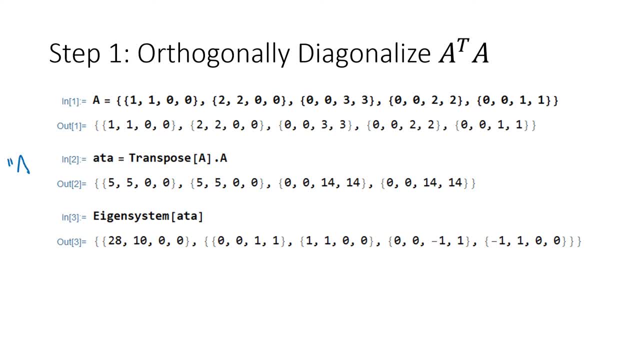 times A, which I just call ATA, because again, this just looks like A transpose A. So just to have an abbreviation for it, I just like to call that ATA. And then we find an eigen system for our matrix: A transpose A. So what we're seeing here is that we've got four eigenvalues. 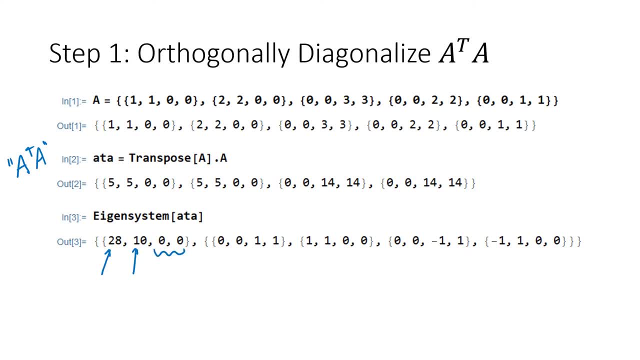 where we count zero twice. So it's a 4x4 matrix. A was 5x4, five rows and four columns, So A transpose A is going to be 4x4.. As we see here, this is a 4x4 matrix. 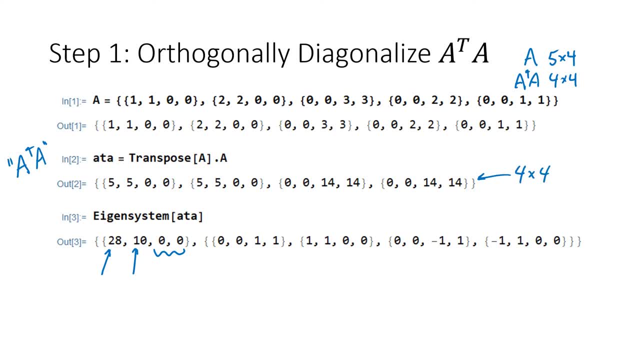 So that 4x4 matrix is going to have four eigenvalues counting multiplicity. So this eigenvector goes with 28.. So if this is lambda 1,, which is 28,, lambda 2,, which is 10,, and this is lambda 3, equals lambda 4, equals zero, this eigenvector goes with lambda 1,. 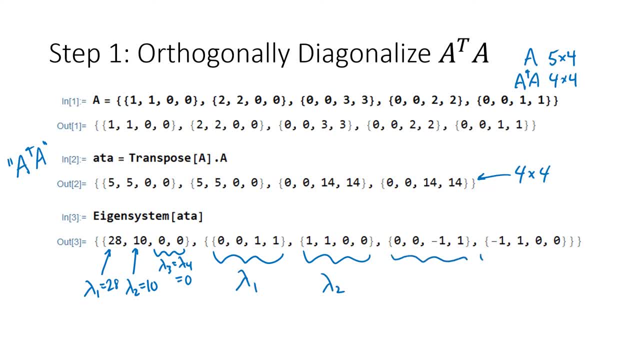 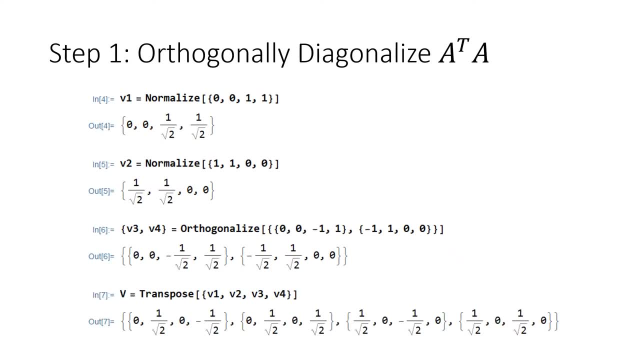 this eigenvector goes with lambda 2, and these two eigenvectors both go with lambda 3, which is the same as lambda 4.. So now we're going to apply the normalize and orthogonalize commands. So for our first vector, our eigenvalue, 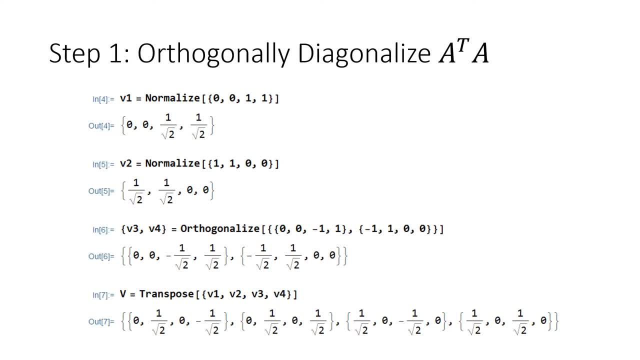 28 just had one associated eigenvector, so we just normalize it. So this vector gets shrunk down to be a unit vector. Same thing with v2, right, So that vector corresponded to our second eigenvalue, lambda 2 equals 10,. 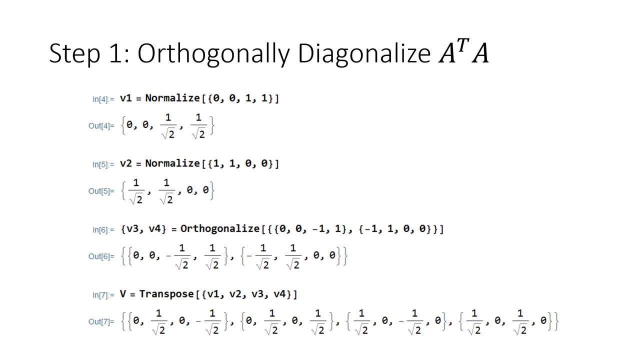 and so, again, we just have to normalize it For our third and fourth eigenvalues, which are both zero. we don't know, just offhand, It does turn out to be true in this case, but in general, the eigenvectors that we get don't have to be orthogonal to each other. 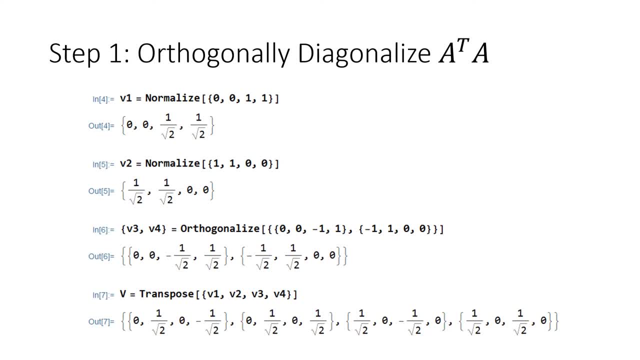 So the way that we can just always apply the orthogonalize command to apply the Gram-Schmidt process and make them be orthogonal. So these four vectors are going to be the columns of my matrix V. So these four are the columns of my matrix capital V that I'm trying to build. 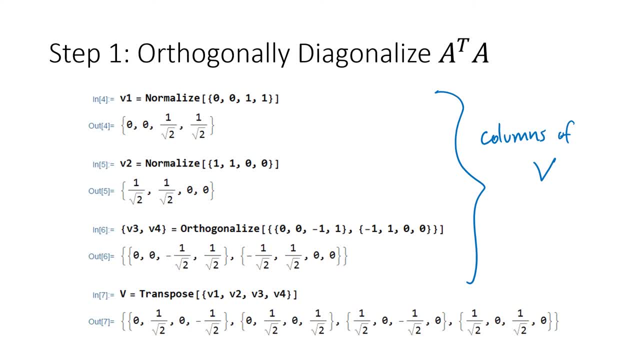 And so the way that I do that in Wolfram, if I just type in v1,, v2,, v3, v4,, if I just type that in, this is the matrix whose rows are these vectors: v1,, v2,, v3, and v4.. 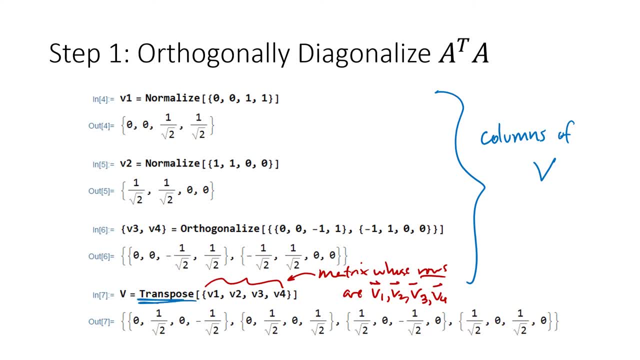 So I'm going to apply the transpose command to change that into the matrix whose columns are v1,, v2,, v3, and v4.. So that's why you're seeing that transpose command in there. So step two is to actually build these matrices: capital, V and sigma. We've already built capital. 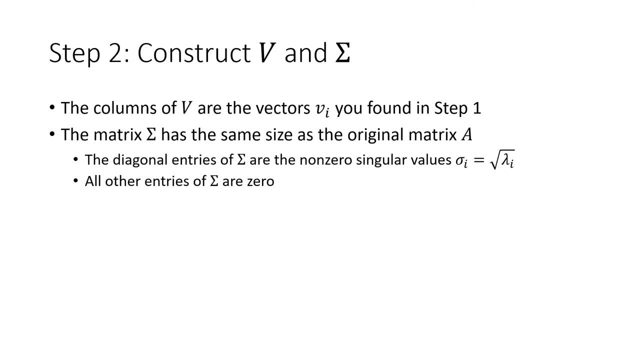 v. You just saw that on the previous slide. Now, what's sigma? Sigma is the matrix that has the same size as the original matrix, a. So remember, a is five by four, So sigma is five by four, The same size. And so what sigma is going to look like is it's going to be mostly zeros. So the way that 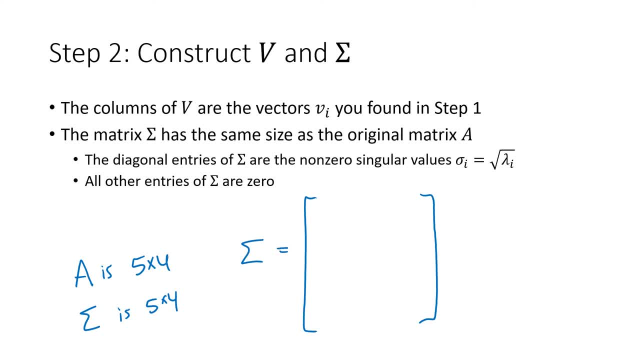 sigma looks is going to be mostly zeros, but the diagonal entries of sigma are going to be the square roots of my eigenvalues. So remember that we had lambda, 1 was 28,. so sigma 1 is the square root of 28.. That's my first singular value. So my upper left-hand corner entry here is the square. 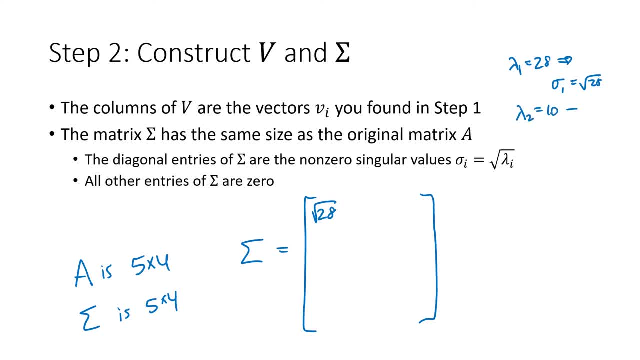 root of 28.. Lambda 2, my second eigenvalue was 10, and so sigma 2 is going to be the square root of 10.. And so I go down and to the right and I get a square root of 10.. Lambda 3 and lambda 4: 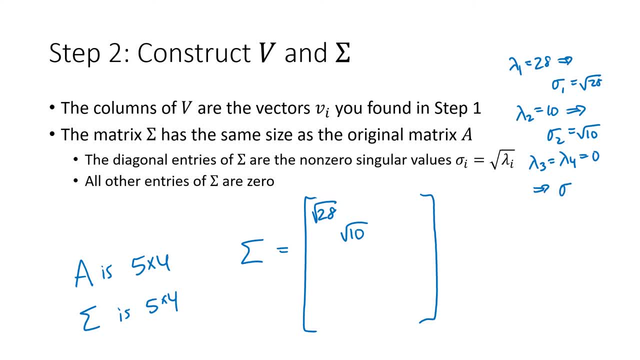 were both 0,, and so that means that sigma 3 and sigma 4 are both 0. So I get a 0 and a 0. And then everything else in this matrix sigma is a big old 0.. 0,, 0,, 0,, 0, 0.. So that's my matrix sigma. 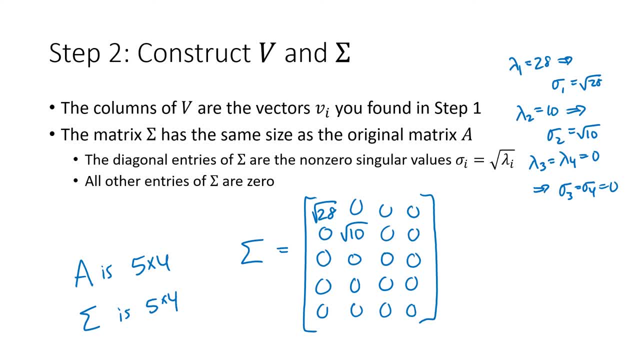 Now if you run out of room in sigma, right? so if you have more singular values than you have rows in your matrix sigma, then you end up throwing out some of your singular values, But, as it turns out, the only ones you'll ever throw out are zeros, so you're not really losing. 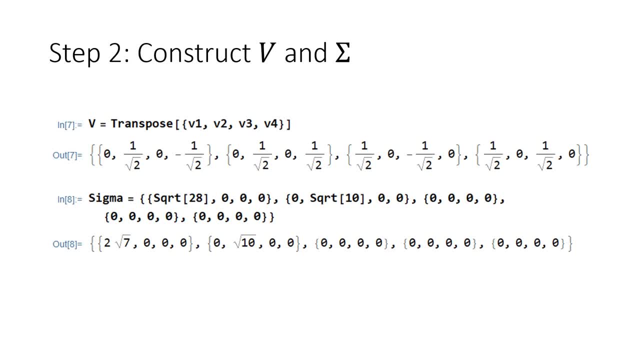 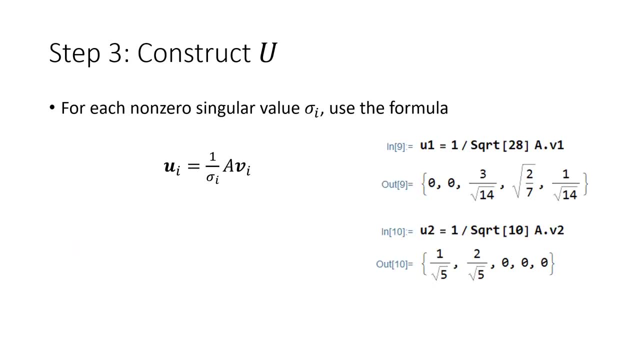 any information. And again, here's how we would type that into Wolfram. We already had capital V from the previous slide, and here's me just typing in sigma by hand: All right, so the third and hardest step here is to construct the matrix U. Now for some of our singular values. we're 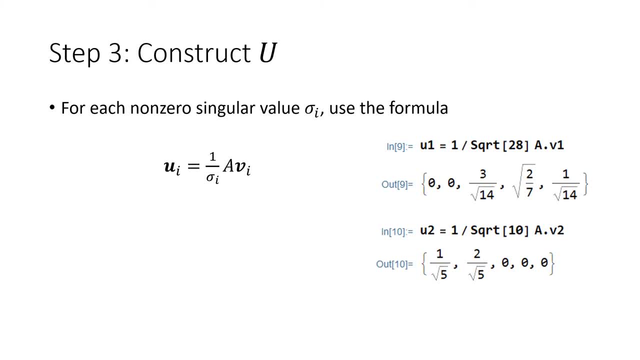 going to do is plug into our formula. Remember that we had: sigma 1 was the square root of lambda 1,, which was the square root of 28,, and sigma 2 was the square root of lambda 2,, which was the square root of 10.. So all I'm doing here is typing those into my formulas and I get two vectors. 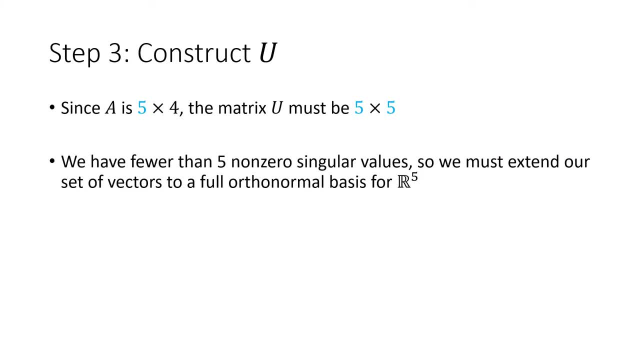 U1 and U2.. Now A is 5 by 4, so the matrix U has to be 5 by 5, right? So the way that this is going to work is: U sigma V. transpose: A was 5 by 4.. Sigma is the same size as A, so sigma is also 5 by 4.. 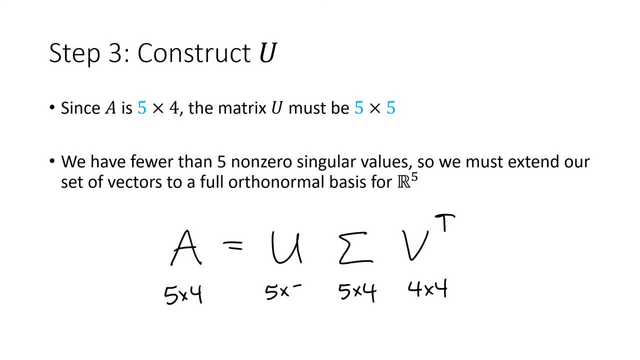 V and U are both square matrices, which means V has to be 4 by 4, and U has to be 5 by 5. And so far we only have two U vectors. We're going to need a total of five U vectors, and so that means that 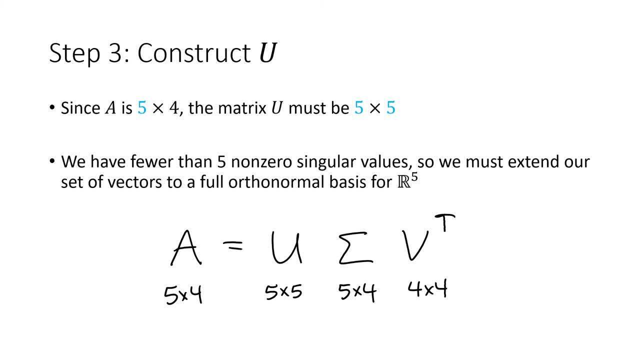 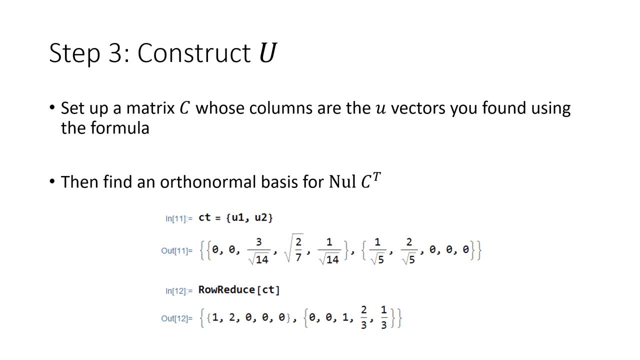 we have to take those two vectors that we've already found and extend them to a full orthonormal basis for R5.. So the way we're going to do this is by setting up a matrix, which I'm going to call capital C. 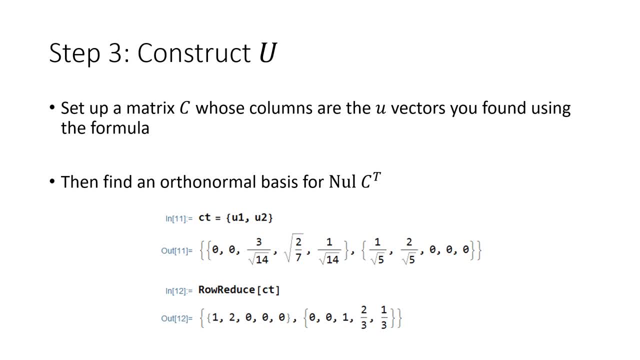 whose columns are the U vectors that we've already found. So so far we've found two vectors, U1 and U2.. So capital C is going to be the matrix whose columns are U1 and U2. And then we're going to take that matrix and flip it around, form the transpose, So C transpose is: 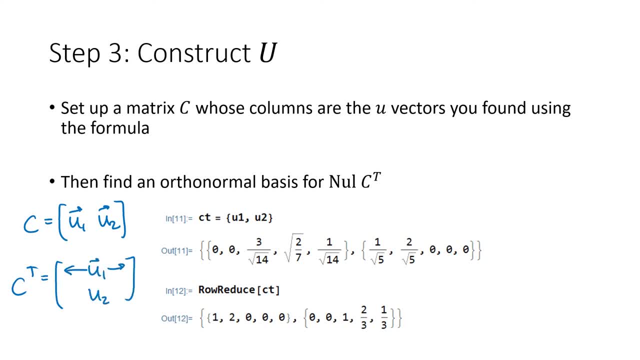 going to be the matrix that has two rows, U1 going across the first row and U2 going across the second row. This is how I enter that in Wolfer. So if I put curly brackets and just start listing, those vectors get written as the rows. So those are my two vectors And now I'm looking for an. 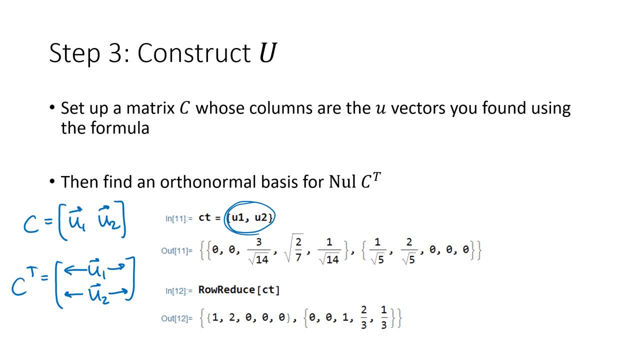 orthonormal basis for the null space of C transpose. So I'm going to row reduce C transpose. That's going to give me 1,, 2,, 0,, 0, 0, and then 0, 0,, 1,, two-thirds, one-third, Remember we're 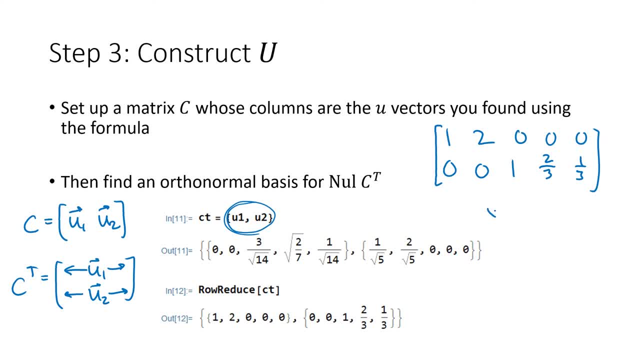 trying to find a null space, which means I need to interpret this as two equations: x1 equals negative 2x2.. x2 is going to be a free vector and x2 is going to be a null space. So I'm going to 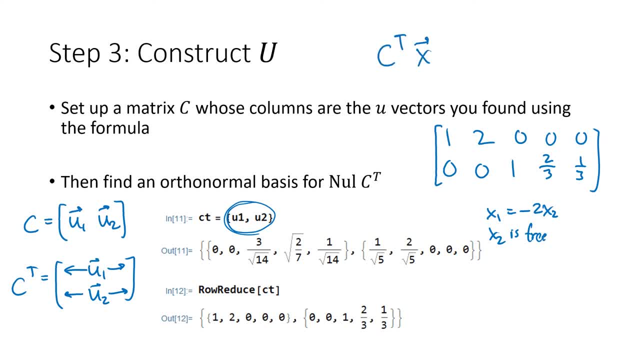 write a free variable. So I'm solving the equation. C transpose times: x equals 0.. That's how I find a null space: x3,. getting back to the second row, x3 is going to be negative, two-thirds, x4, minus. 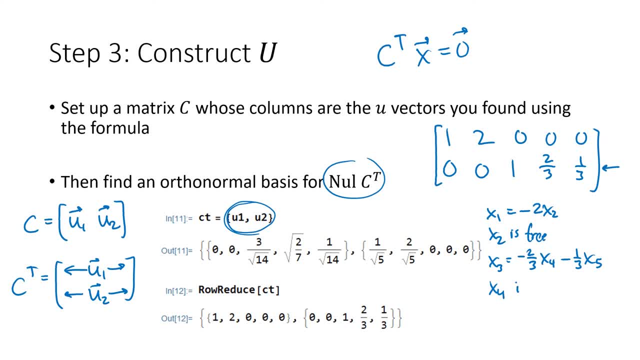 one-third x5. And then x4 and x5 are both free. Since I need a basis for this null space, I need to write this solution in parametric form. So here's what that parametric form looks like I get. 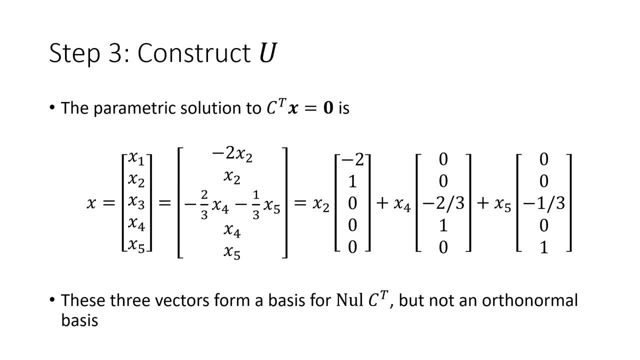 three vectors, and those three vectors form a basis for the null space of C transpose, but it's not generally going to be an orthonormal basis. Again, the problem needs to be that these three vectors have to be all unit vectors, which they're clearly not, and they all have to be orthogonal to. 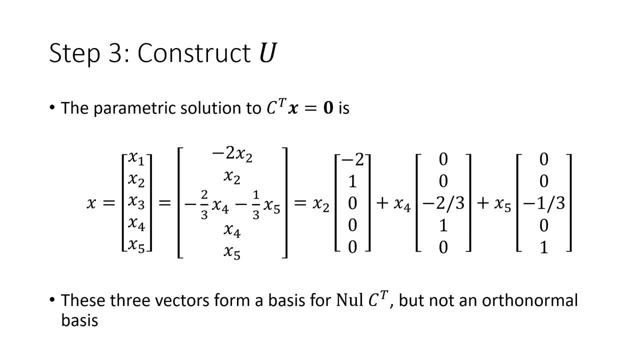 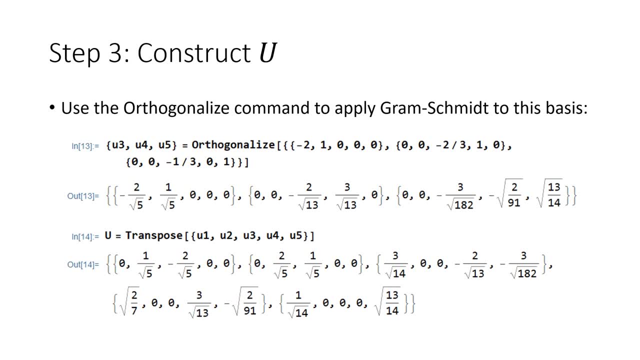 each other, which is also not true. So the way that we fix both of those problems is by using the Gram-Schmidt process, again using the orthogonalized command in Wolfram, And here's what that looks like. So we type in our three vectors, so this, this and this and this.